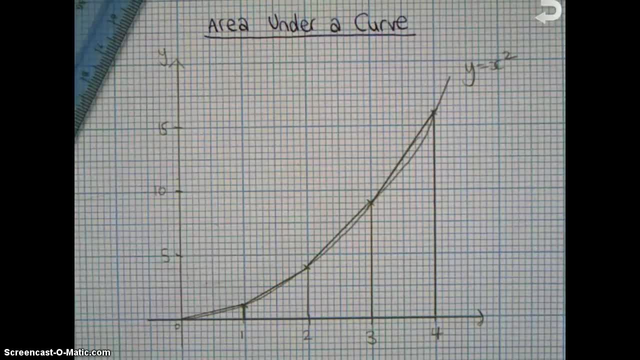 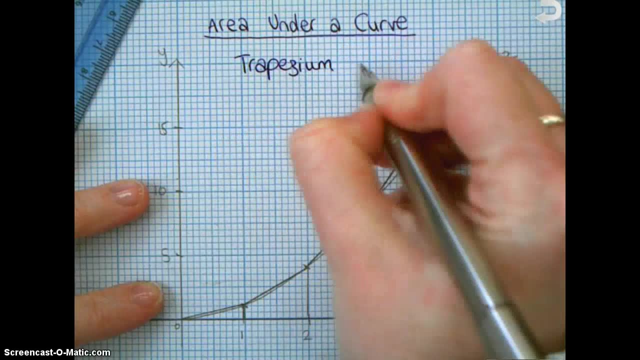 So all we do for this area under a curve, the method that we're using, or what this is called, that we're about to do, it's called the trapezium. So what we do is we say, if I look at each of these trapeziums separately, 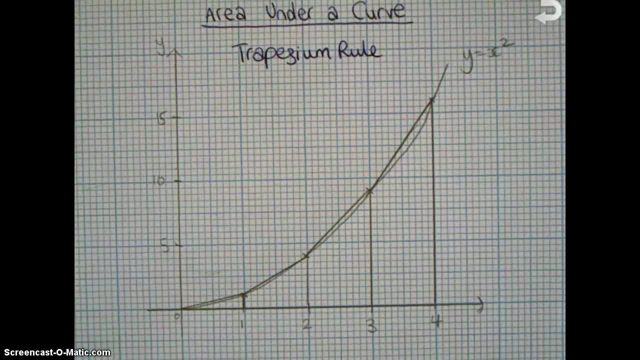 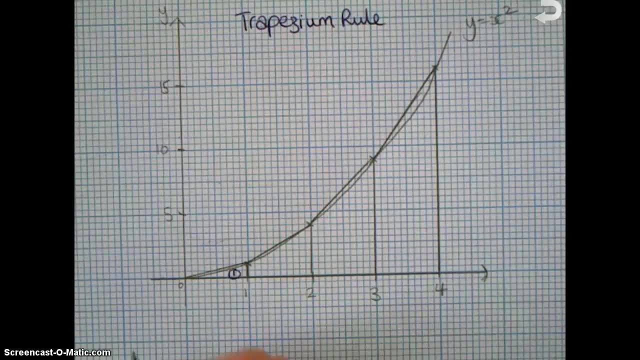 so I've got 1,, 2,, 3,, 4, and I work out the area of each one individually. So trapezium number 1, I'll say the area of that trapezium- is the sum of the parallel sides. 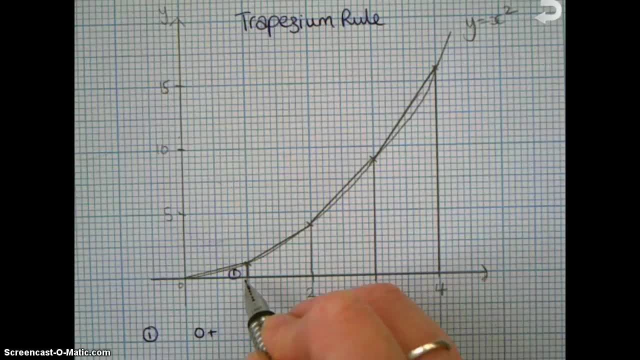 so this parallel side is 0, plus the height of this side. well, 1 squared, that goes up as high as 1.. So it's 1.. So that's 1, plus 1, 0 plus 1, divided by 2, times by the height. 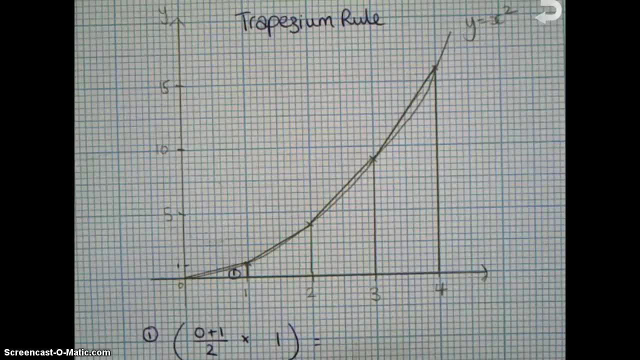 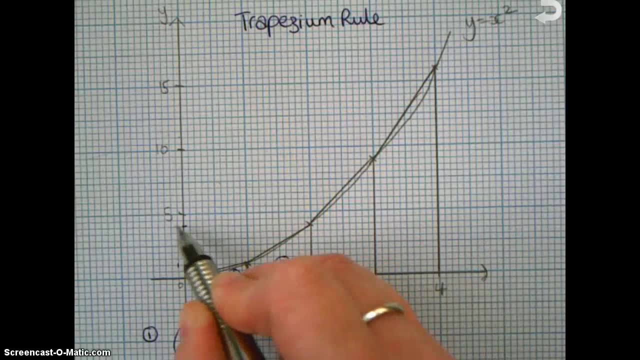 the distance, there is my 1. And that will give me the area of that trapezium, Trapezium number 2, that's this one. well, that will be. this side is 1, that height, 2 squared, that goes up as high as 4, doesn't it? 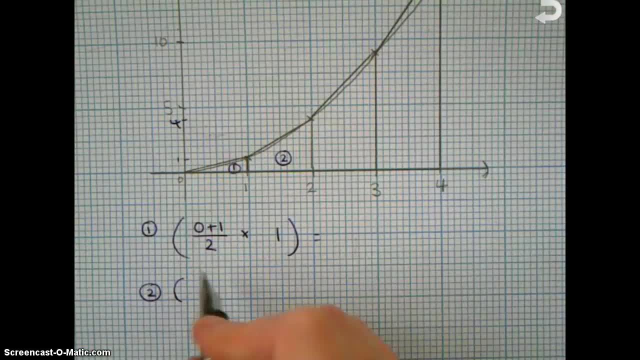 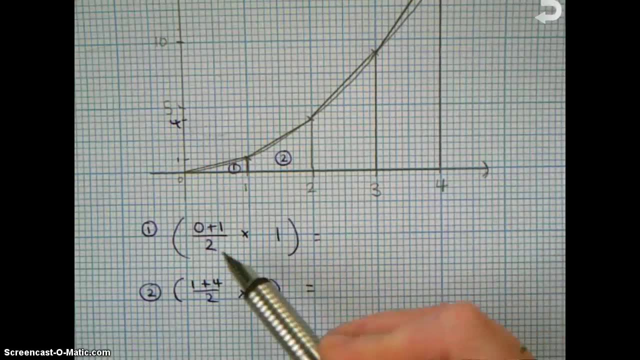 So if we're working out our second trapezium, we're going to do 1 plus 4 divided by 2 times 1.. Sorry, I could work these out, couldn't I? So that's: 0 plus 1 is 1, divided by 2 is a half times 1 is a half. 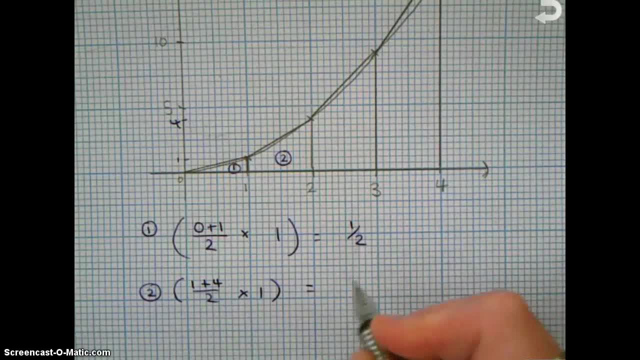 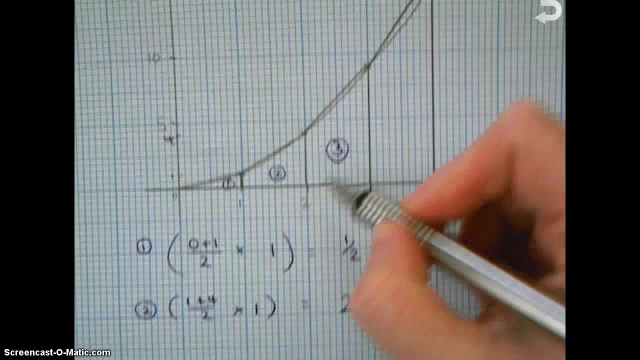 1 plus 4 is 5, divided by 2 is 2 and a half. times 1 is still 2 and a half. Do the same for trapezium 3.. This height's 4, this height up to here is now at 9.. 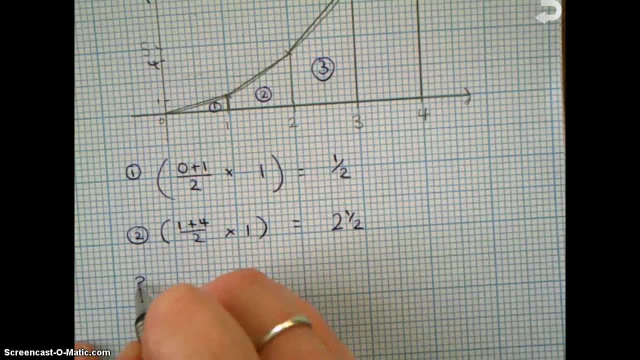 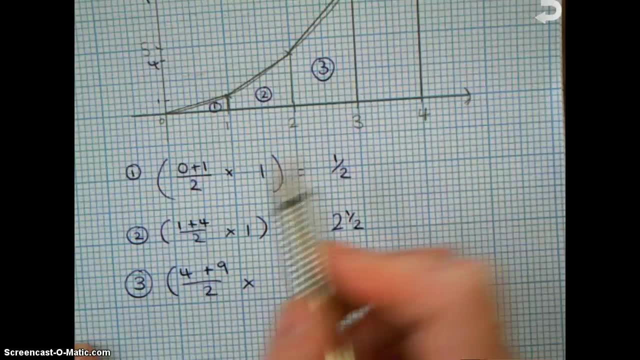 So that rule for trapezium 3 is going to be 4, add 9, divided by 2, times the height of the, All of these trapeziums are 1,, aren't they? Because it's the width between our spacings. 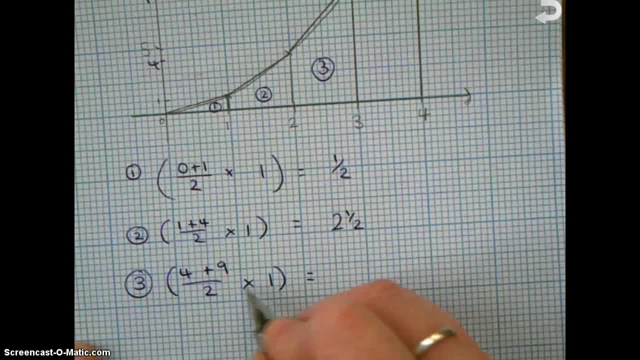 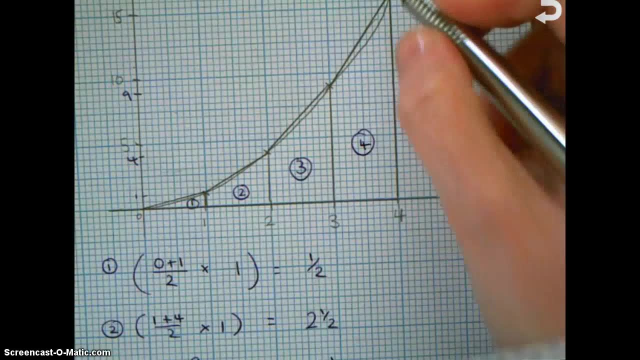 So 4 add 9 is 13,. divided by 2 is 6 and a half times 1 is still 6 and a half. And we do the same for the last trapezium. This height's 9, that point goes up to 16, at the top up there.